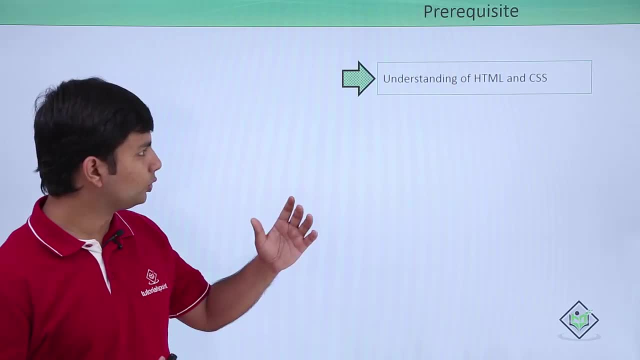 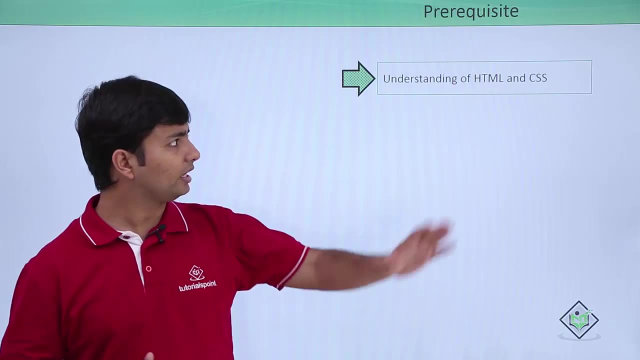 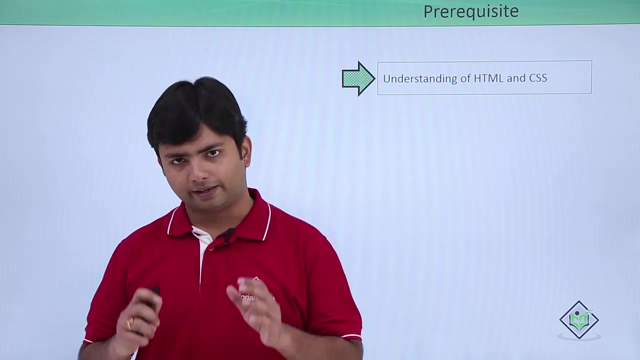 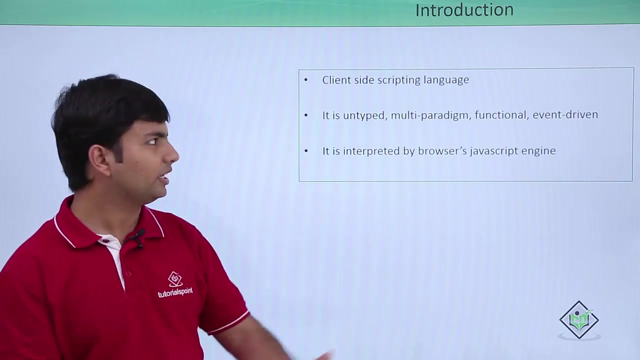 So make sure, before getting started with the JavaScript, you have the sufficient knowledge of HTML and CSS, as we will be working with the web page, and these two are the important things which you must know for creating the interactive web page. Now here, as I just said, it is a scripting language, but if I add something more, I will say it is a. 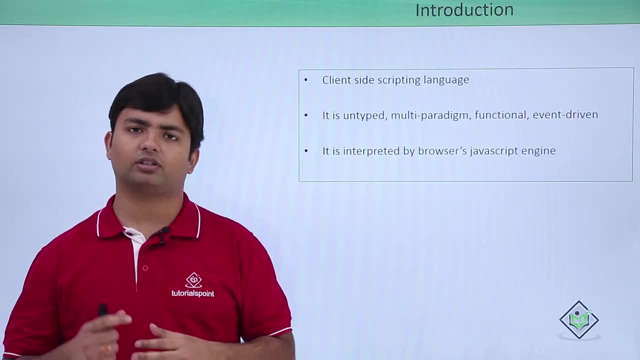 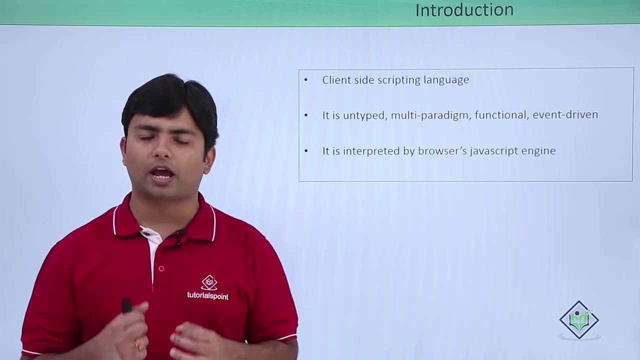 client-side scripting language. Client-side means: whenever you will execute the JavaScript on a web page, the complete execution will happen on the client-side only. There will be no server-side interaction while executing the JavaScript. That's why, whenever we will try to do the JavaScript on the web page, we will not be able to execute it on the client-side. 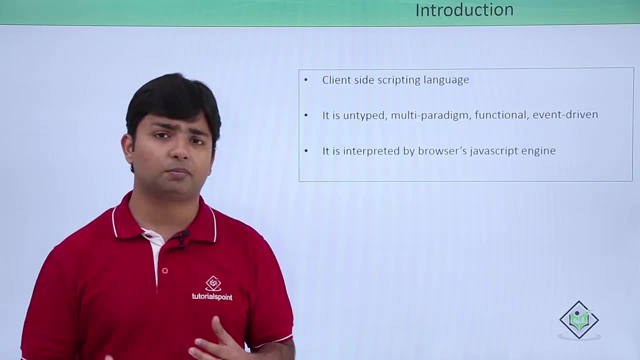 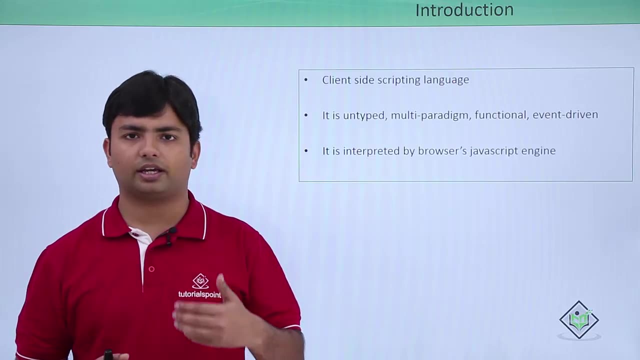 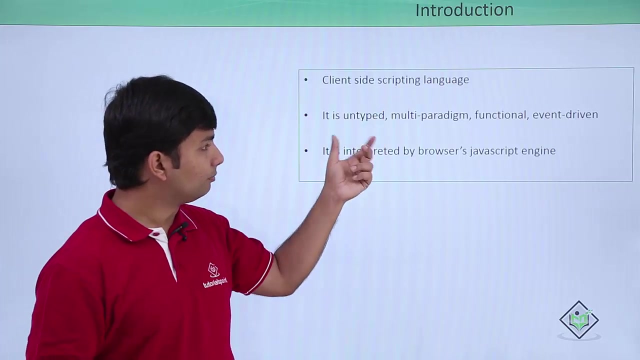 So if we do some operations like putting the validations or doing the animation, like things, everything will execute on the client-side, which will also efficiently execute the page, means the performance of the page will be more better. Now something more about JavaScript. let's see, it is untyped. Untyped means if we know something. 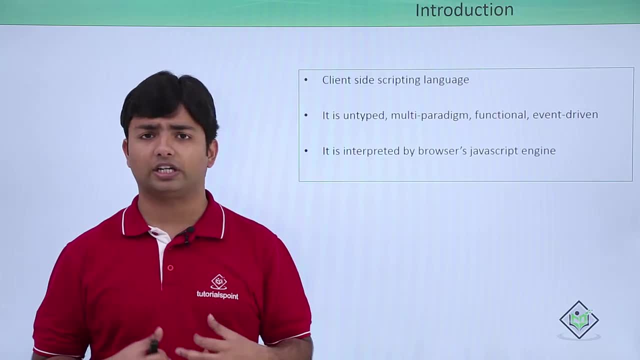 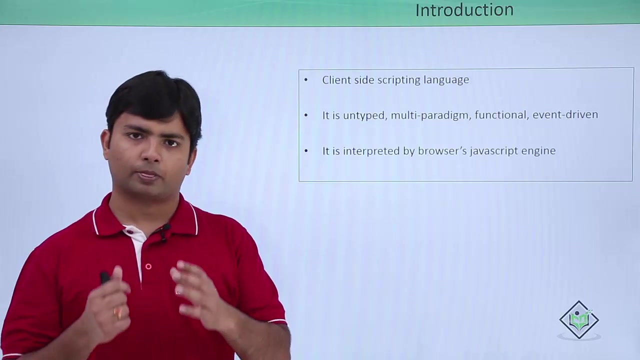 about the programming languages. you may know about the thing called data types, which specifies the type of data we are going to process, But while working with JavaScript you will observe like it is untyped means it is not a type-safe language. So whenever you will have to store, 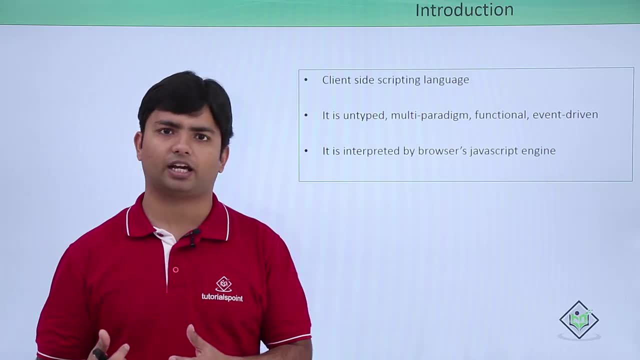 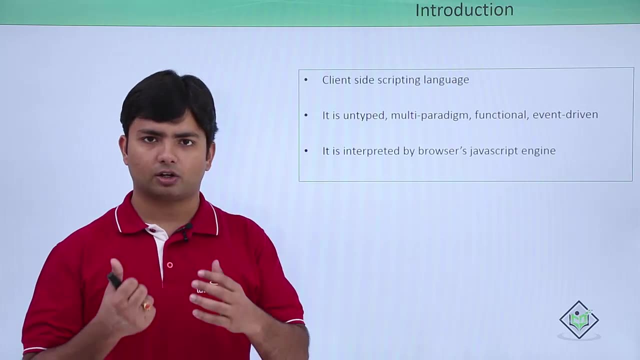 something. you will just use a variant type, and that type can store any type of value, So we will have to take care like which type of data we are going to manipulate manually. Apart from that, it is multi-paradigm, So we will have to take care like which type of data we are going to manipulate manually. Apart from that, it is multi-paradigm. 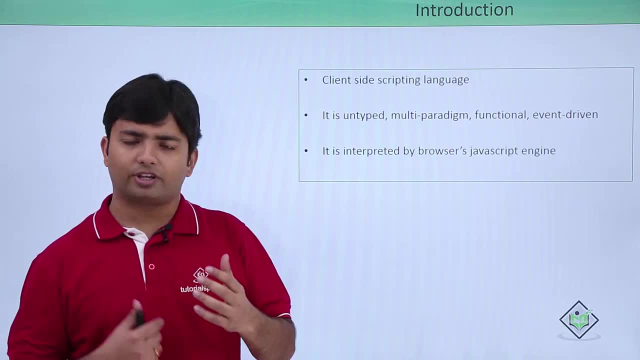 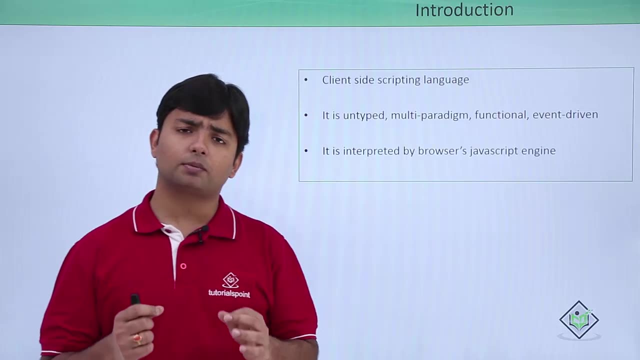 So we will have to take care like which type of data we are going to manipulate manually. Apart from that, it is multi-paradigm Means you can do various kinds of development, website development, things related to JavaScript. Nowadays, JavaScript is also a backbone of so many different technologies like jQuery, AngularJS. 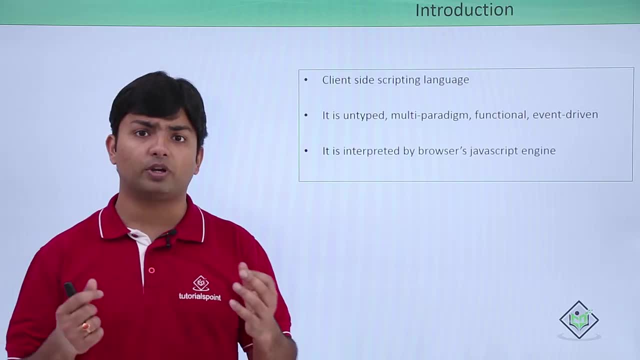 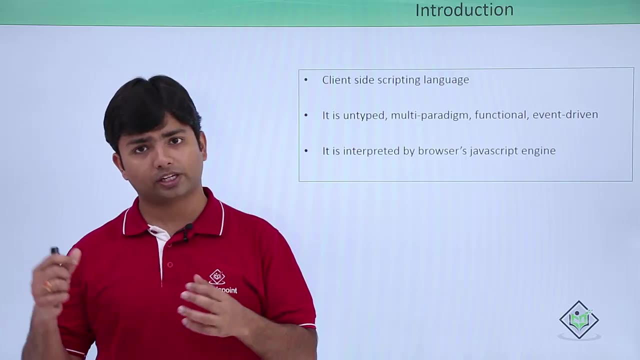 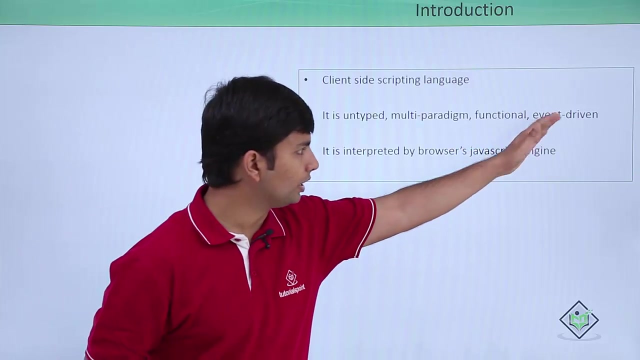 NodeJS and so many JS-like technology you may be hearing nowadays. It is functional, which will make the code even more modular. You can split the particular code in the different functions And you can call them up on a particular event, as it is also event driven. So 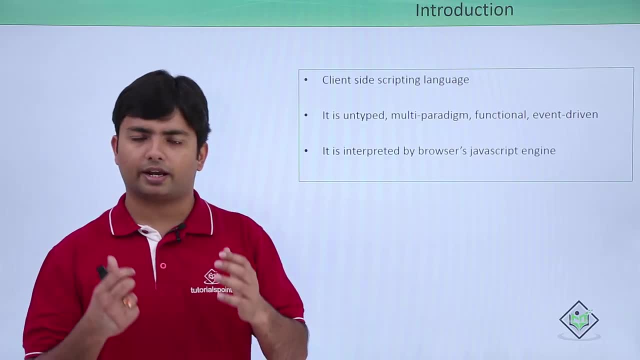 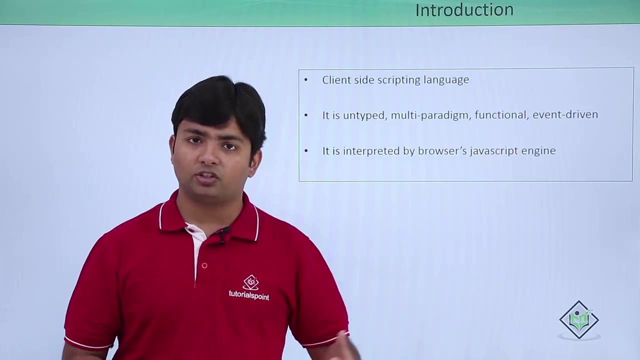 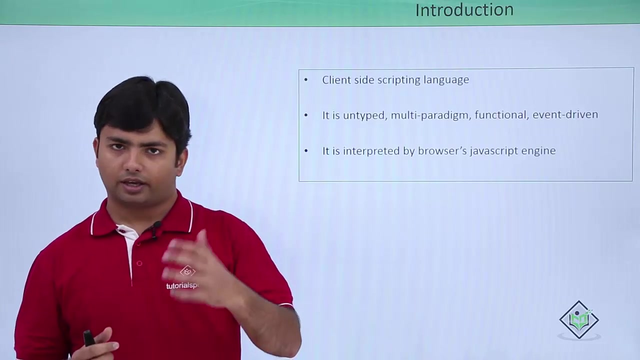 using JavaScript in such a way will make it wonderful, and so that we can use it even more creatively. It is interpreted by browser's JavaScript engine. Now, if the question comes, like when I write a simple HTML, how it runs, Every browser has a parser which reads the HTML tags and 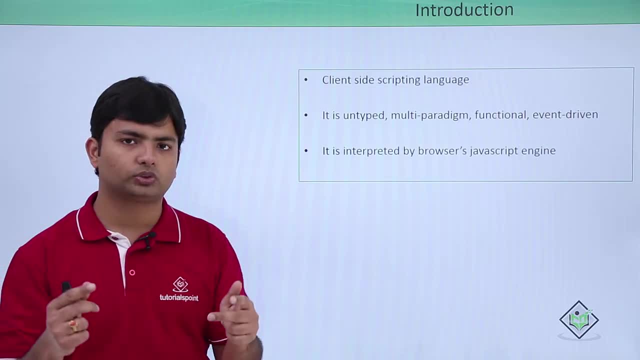 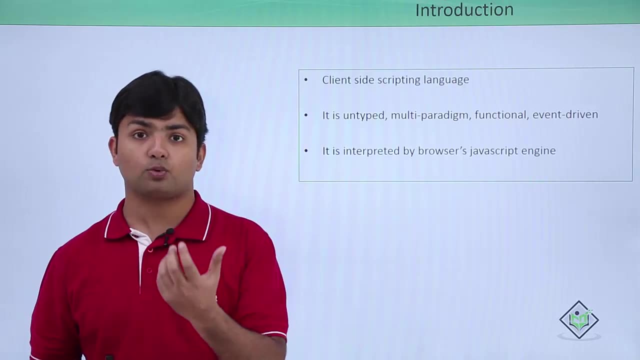 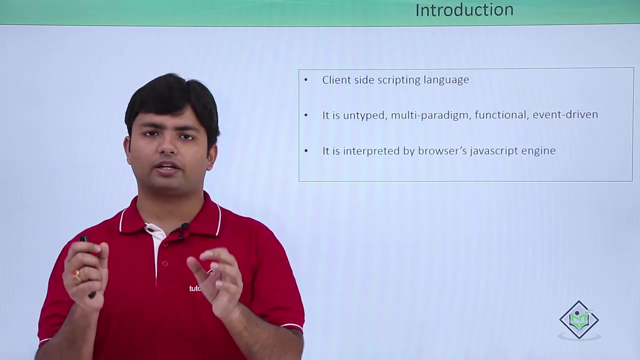 render the text accordingly. For example, if I use H1 tag, so the text written within the H1 would be shown as the H1 as a heading 1, the biggest heading. But if I say what about? JavaScript means if I am writing some logical code, some programming-like code, how the browser will. 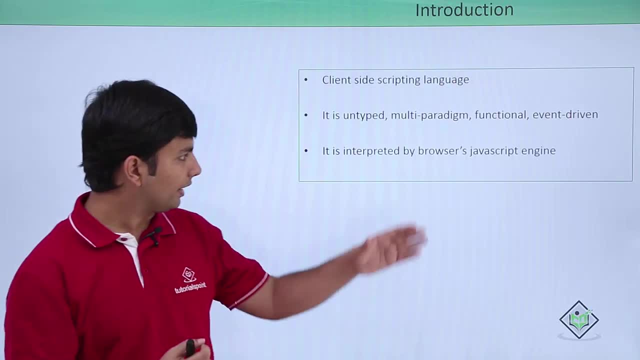 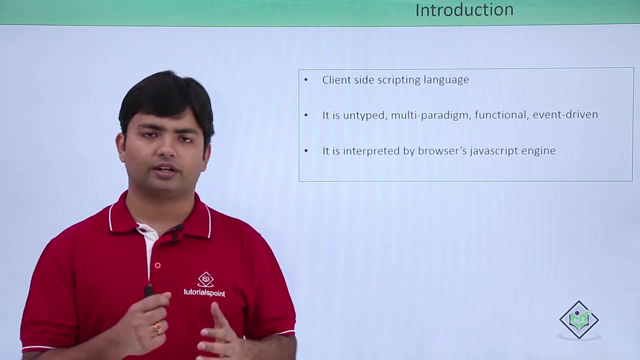 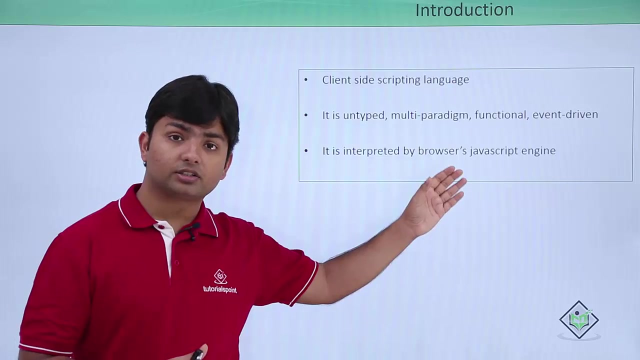 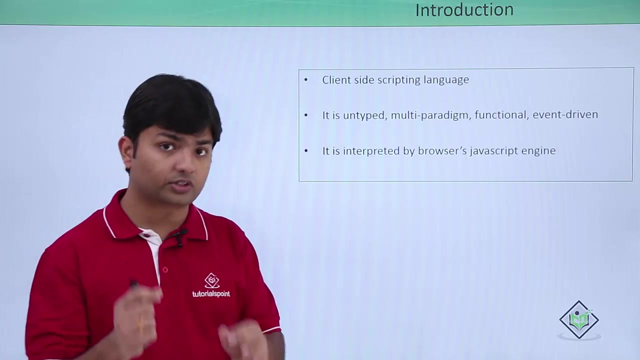 be able to execute that. So for that, as it is mentioned, every browser has the JavaScript engine. for example, for chrome it is v8 engine. for different browsers it's different engine, so that javascript engine is actually an able enough to execute the code which is run, which is written. 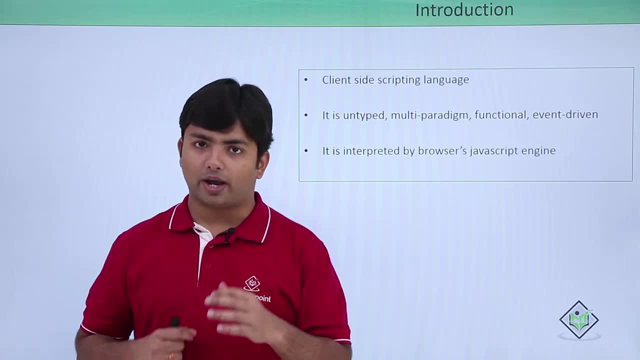 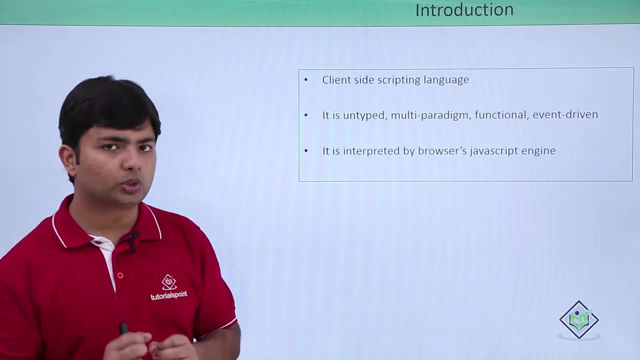 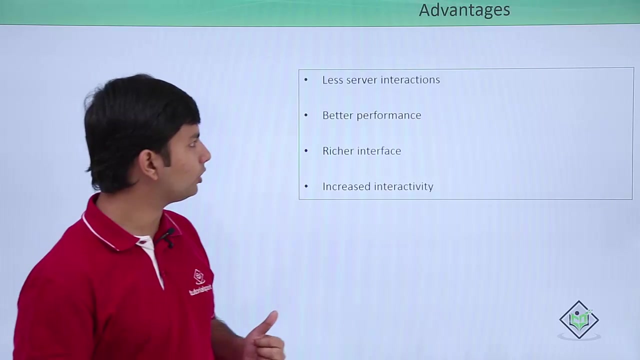 in the javascript and make sure, while doing this, your javascript must be enabled for that particular browser. only then you will be able to see the execution of your javascript code. now let's move on to some more advantages of javascript, as it is less server interaction, all right means while. 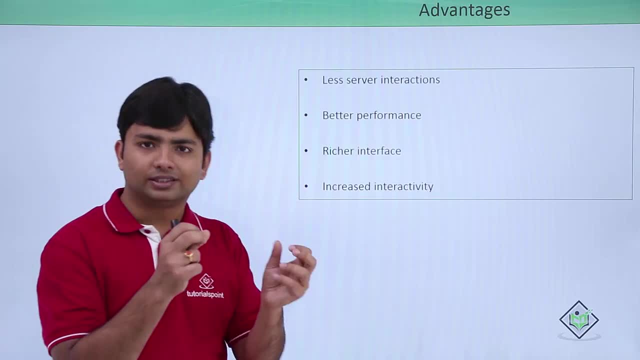 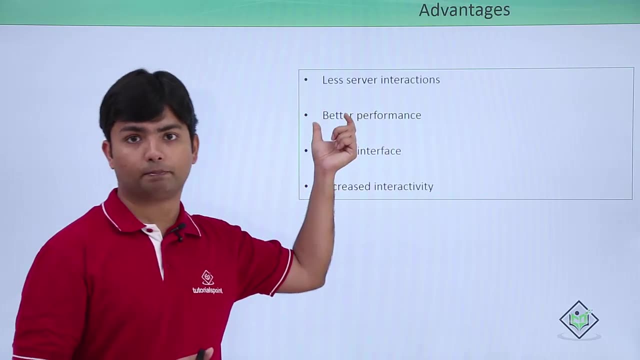 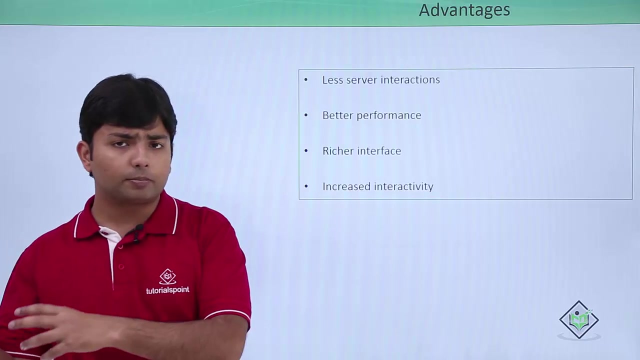 executing. it will execute mostly on the client side, so it will be a lesser interaction with the server, and that will make the performance better. all right, because if the code is here only and it is running on the client side, the page will not be posted back to the server again and again.